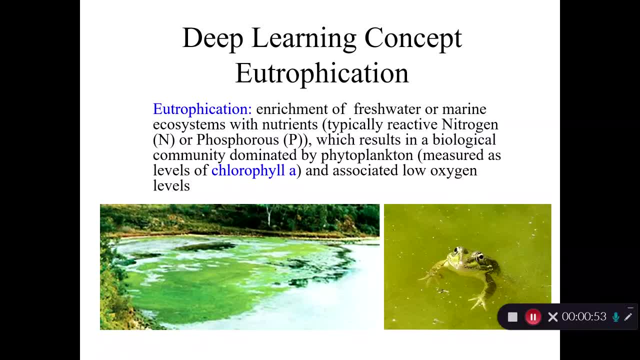 that happens. So, first of all, to define our terms. So when we're talking about eutrophication- eutrophication of aquatic systems- we're talking about what happens in our freshwater and marine ecosystems when they get very high levels of nutrients coming into these, And we'll see that. 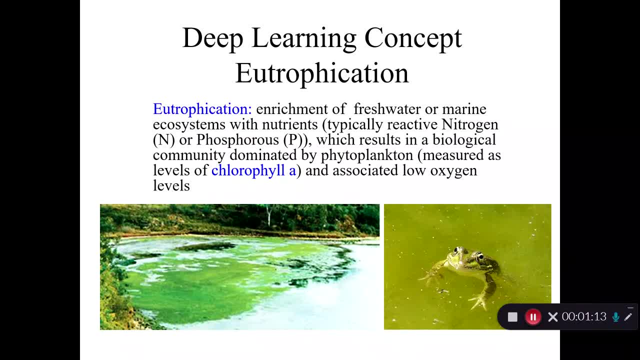 these nutrients can be grouped into two big categories: those that are reactive forms of nitrogen and then also phosphorus. And when you have eutrophication occur, what happens is you get an aquatic community that becomes dominated by phytoplankton. We measure that by: 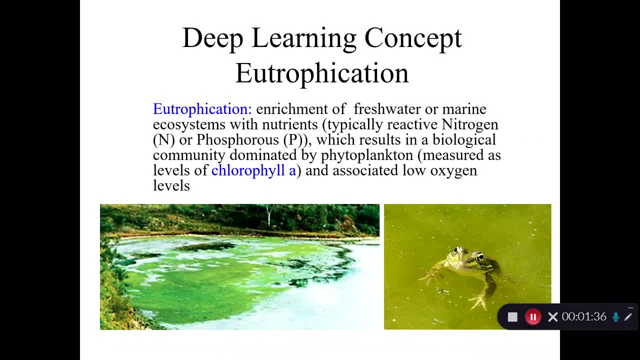 looking at a little bit of water and seeing how much chlorophyll A is in it. So that's a pretty easy thing to do with absorption. And the other thing that happens when we get these high phytoplankton communities is our oxygen levels plummet, And we'll look at why that happens. 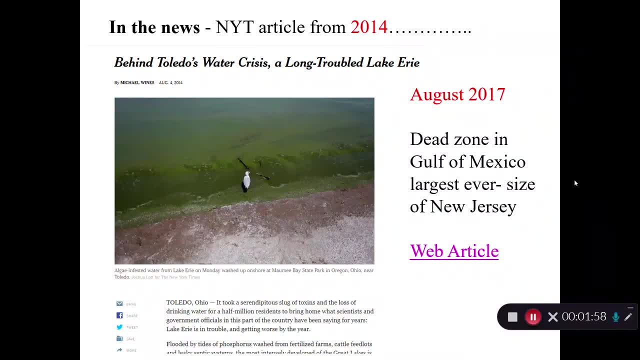 Why is this an undesirable state? to go from this clear water, low phytoplankton system to very turbid water, high phytoplankton. Well, in some cases it can actually have a negative impact on the water supply and make it, depending on what type of bloom you get. 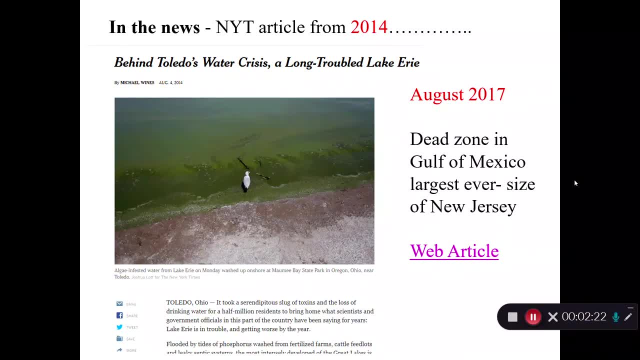 in your plankton community. you can sometimes have toxins in the water that create a lot of water crisis situation because it's affecting people's water supply. So this is just some news articles associated with that, like this New York Times article from 2014, when this 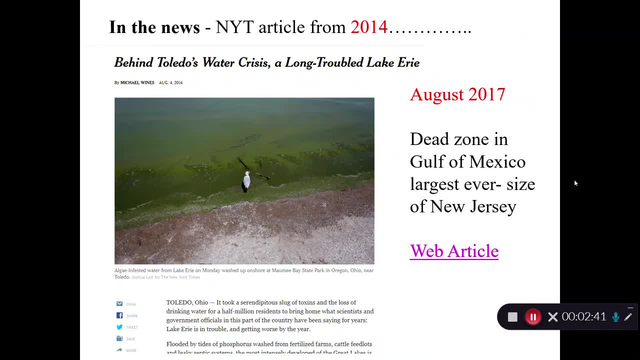 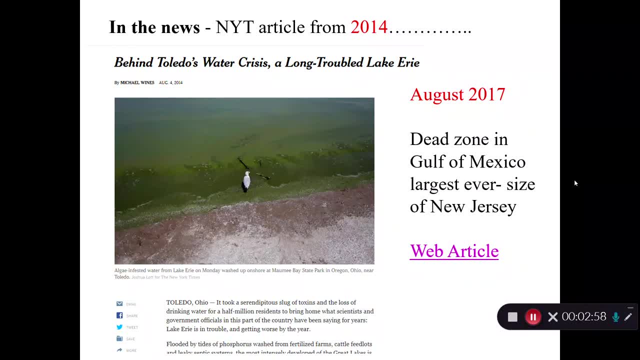 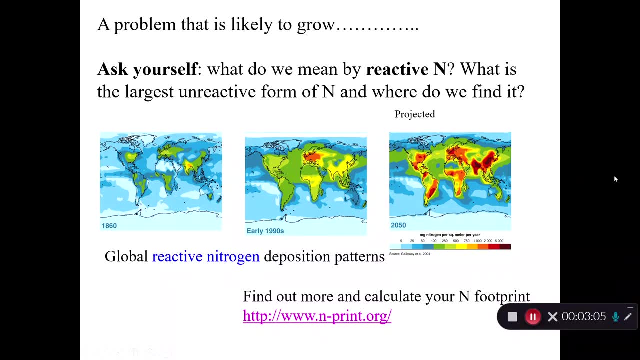 very, very large, to getting to the size of even a whole state. Part of why I'd like to cover this process early is: this is a growing problem And in this pattern here we can see the global patterns of reactive nitrogen, both historically and then projectively. 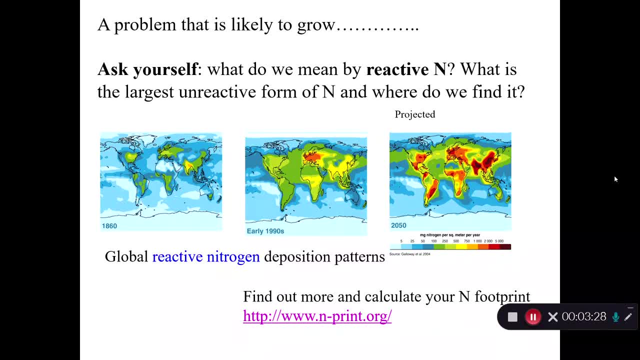 And so what you can see is the historic low levels of nitrogen in our marine systems and our terrestrial systems, and then the projected these very high levels. And I want you to ask yourself a question, right? So we've talked about how reactive nitrogen is one of the groups of nutrients that can. 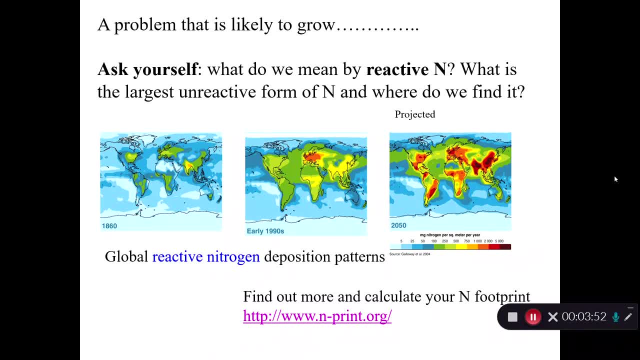 cause these eutrophication events. So I want you to try to think back to chemistry- Okay, Sure, chemistry, or maybe you're in chemistry right now. I think about: okay, what do we mean when we talk about reactive nitrogen, And then maybe it will help you figure out the answer to this question. 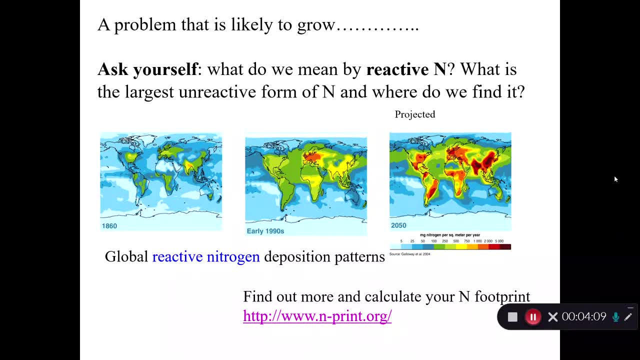 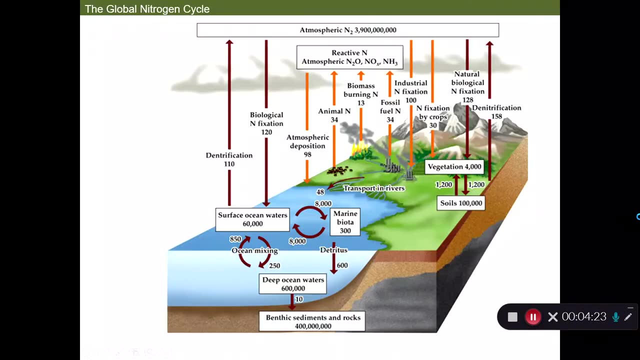 to also think about what is an unreactive form of nitrogen and where do we find it? So take a deep breath And yes, that is a clue- And think about that question And when you're ready, we'll go on to the next slide. So this is one of our biogeochemical cycles. This is our nitrogen cycle. 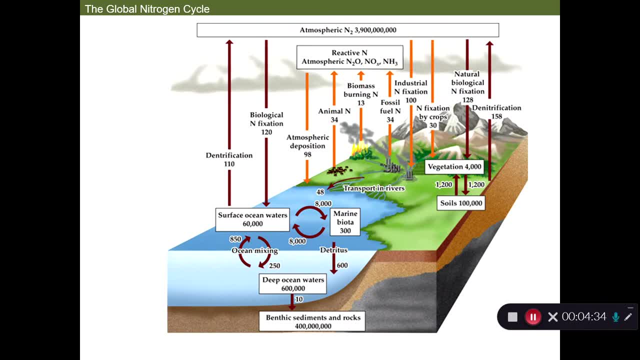 As you can see, it's pretty complicated, And the other thing that you can see in here is that we've really modified it. The ways in which we, as humans, have modified the nitrogen cycle are shown in the yellow arrows here, And what I'd like you to pay attention to right now. 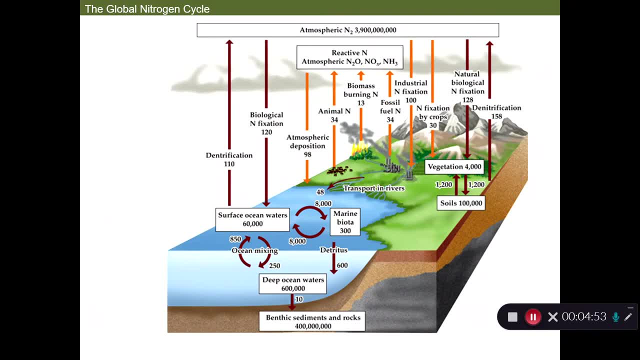 is the nitrogen cycle, So this is one of our biogeochemical cycles. This is our nitrogen cycle, just the atmospheric component of the nitrogen cycle, because it'll help us orient when we start to think about what we mean by reactive versus unreactive. 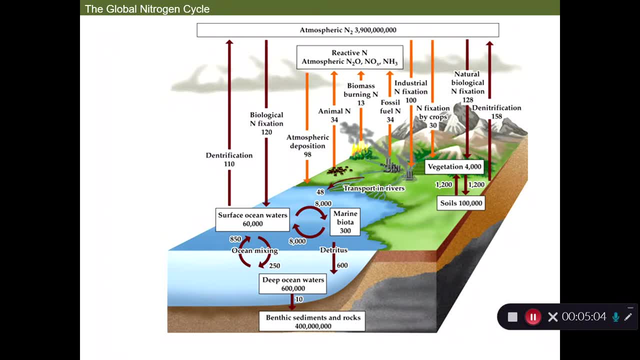 nitrogen. So the first thing I want you to see is that huge amount of nitrogen in the atmosphere. So the nitrogen cycle is known as an atmospheric cycle because there's so much nitrogen in the air, and that's why I ask you to take a deep. 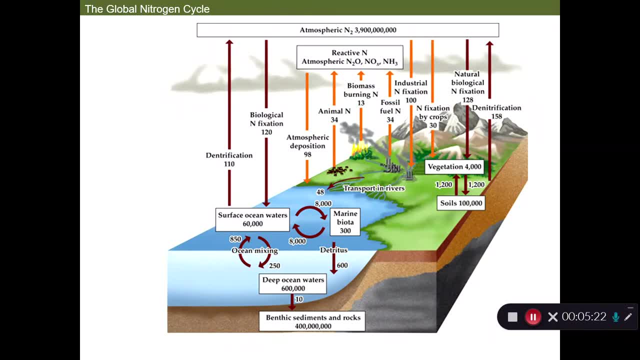 breath Right, because be like: oh yeah, I'm breathing in mainly nitrogen, So 78% of the atmosphere. you can see there's a huge pool of nitrogen there, but it's in that form into nitrogen gas that's very inert. The reason why is: 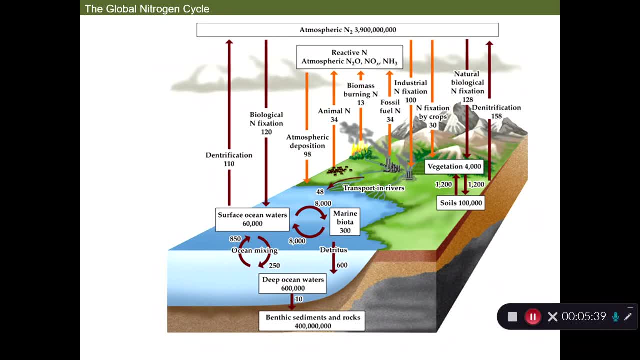 those two nitrogen atoms are held together with a triple bond that's really really hard to break. So this big pool of atmospheric nitrogen, it's very inaccessible. it's a very inert form. Then you can see if you go just one box down in the nitrogen cycle. one thing that we have done: we have these yellow arrows feeding into that box where it says reactive nitrogen. 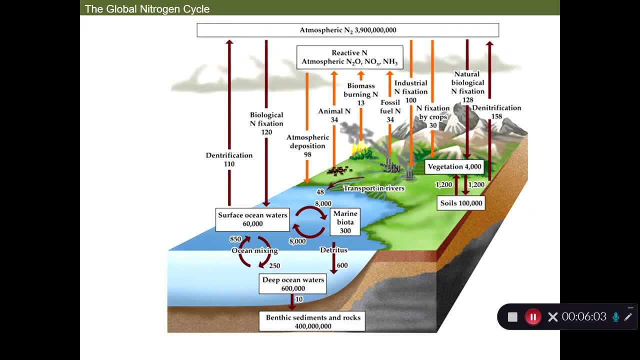 And then it has some of our various forms of reactive nitrogen listed, right, like our nitrous oxide and our ammonia. And then, of course, we could also think of our nitrates and our nitrites and our ammonia, ammonium, all of those. 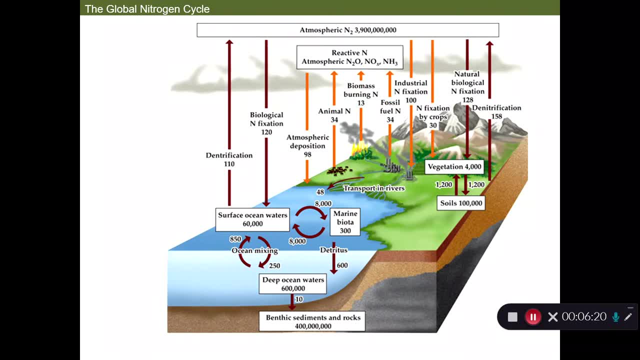 So basically all of these forms where you attach either some variety of oxygens to it or some variety of hydrogens. So you can start to see why we also have the term reactive nitrogen right, because once we move from that inert form it can actually have a lot of different forms that are reactive. 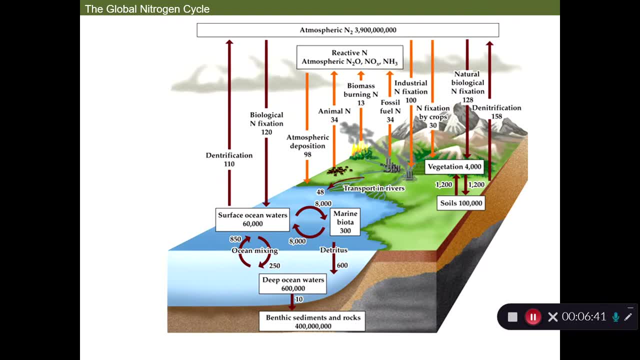 So we've clearly made more reactive nitrogen in the atmosphere. The other thing you'll see on here is a yellow arrow coming down from the atmosphere That says industrial nitrogen fixation. So what we're doing there is we're making fertilizer right, So we pull that nitrogen out of the air. 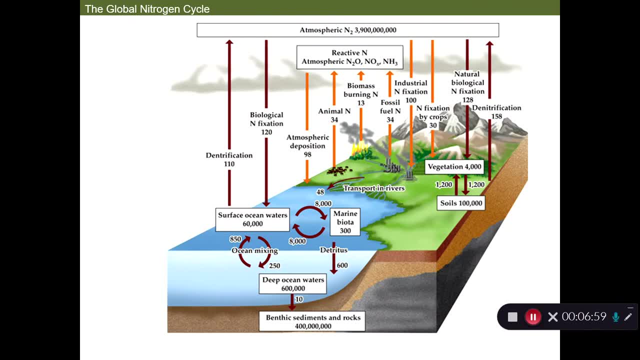 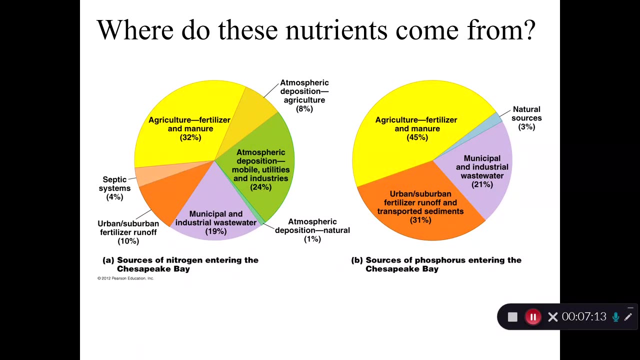 We combine it with hydrogen gas- high temperature, high pressure- and we make reactive forms of nitrogen that we put out on our fields. All of us are familiar with the big white tanks out on the cornfields here in Illinois. Well, it turns out those big white tanks out on the cornfields impact our stream system. 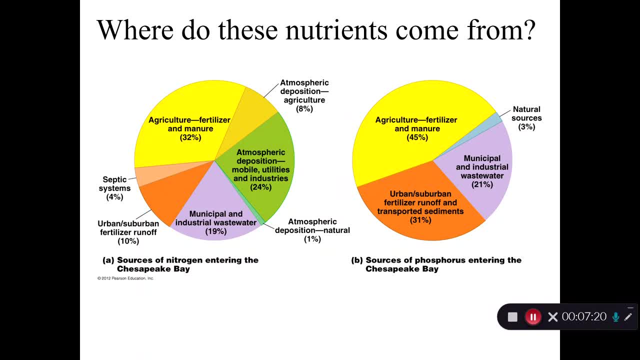 And our ocean systems. So this is looking in particular at first nitrogen and then phosphorus, and where are they coming from before they hit the Chesapeake Bay on the East Coast, And so you can see that fertilizer for agriculture is a big piece of where those increase in nutrients to our aquatic systems is coming from. 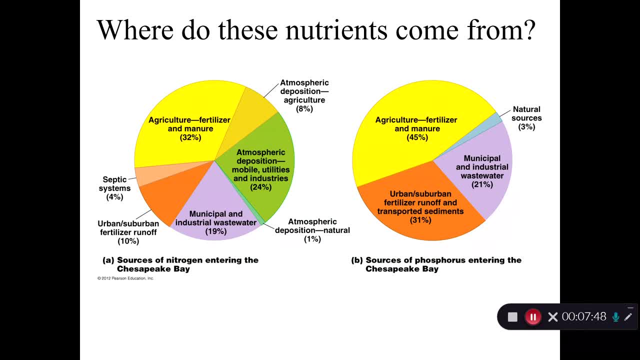 And you'll see that for nitrogen And in particular, we already talked about how we create more reactive nitrogen in the atmosphere. So you can see that big green slice to the pie too, suggesting that another big source of nitrogen for the bay is that atmospheric deposition. 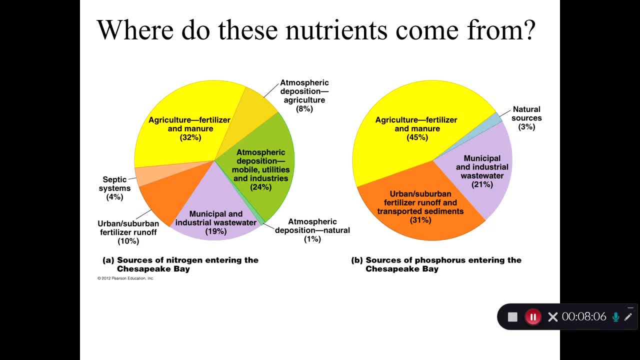 I will say that burning fossil fuels is one of the things that creates that. So we have a variety of sources in our landscape and because of how we modify things with fossil fuels, we can create a lot of that fuel use and fertilizer use that make it so that there's more reactive nitrogen. 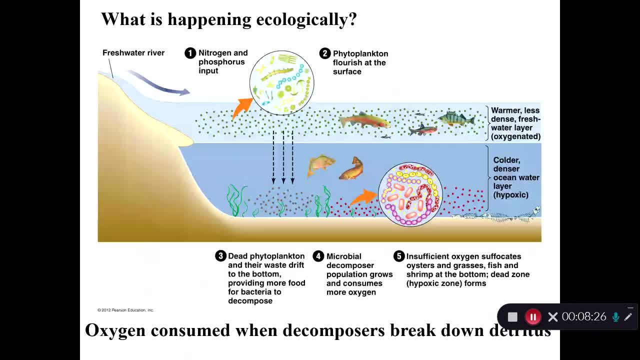 and more phosphorus coming into our waterways. So what then happens ecologically when we get nitrogen or phosphorus coming in to a system? Well, here we have freshwater river coming into a lake or ocean and the first thing that happens is you get that bloom in the phytoplankton. So it makes sense that 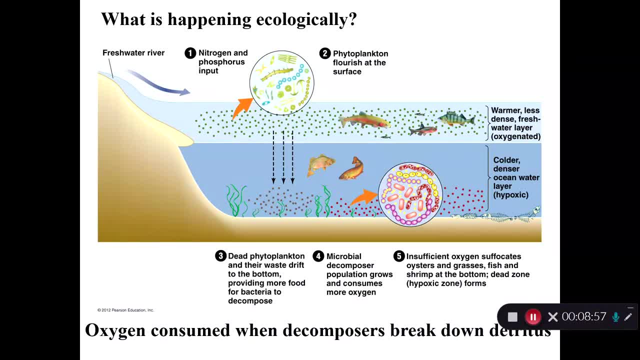 because nitrogen and phosphorus. they're basically like plant fertilizers, right? So when you increase the amount of them in your lake, all of the phytoplankton will flourish. What that means is that you'll get a big buildup of the of that algae, if you will, and as that biomass increases, you also have a lot. 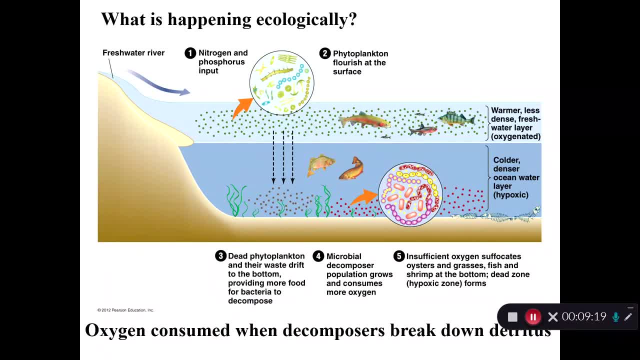 more dead algae right And that will float down to the bottom of your lake. As that biomass accumulates, you start to have what's called a high demand for oxygen in the system, and that's because your decomposers are going to be. 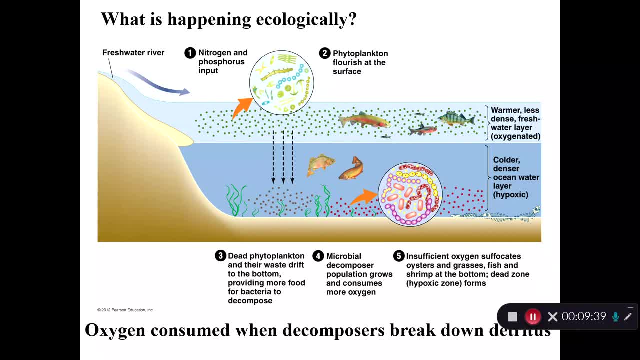 consuming oxygen as they break down all of that nitrogen, And that's because your decomposers are going to be consuming oxygen as they break down all of that dead organic matter that's being produced by the phytoplankton. At some point that oxygen demand can become so high that you don't have enough oxygen. 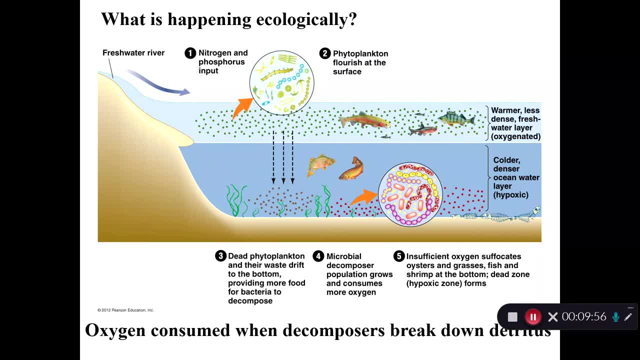 in the system to support your species that need higher oxygen levels, right? So this could be your fish or your shrimp if you're in the marine system, and then you get these low oxygen conditions and then your fish and your shrimp and your other invertebrates start dying. 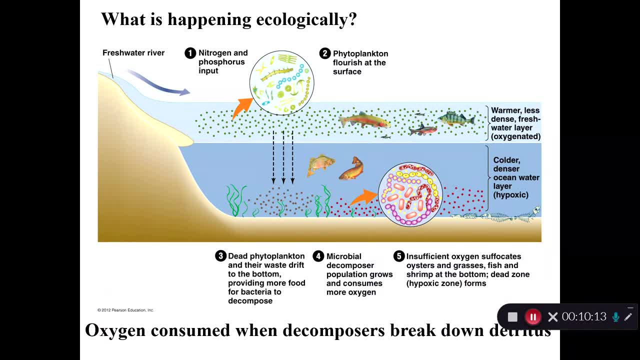 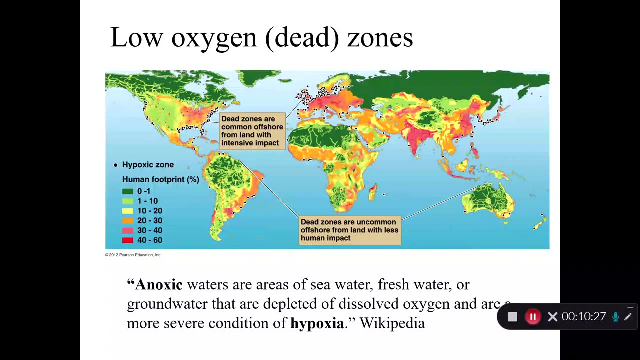 now you've got even more dead organic matter and you end up with an ecosystem that's very high in phytoplankton, very high in dead organic matter, very high in decomposers and very low in oxygen. These are what are called the dead zones. It's 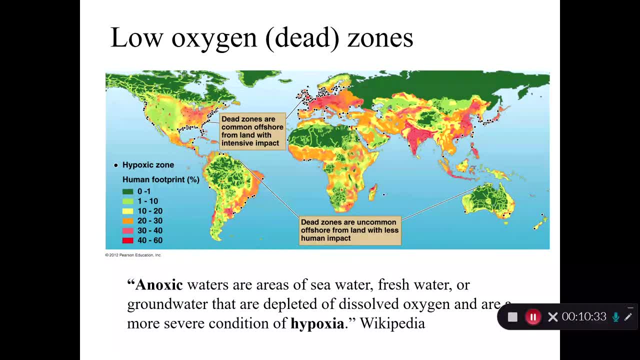 a little bit of a misnomer, because it's not as if things aren't living there, but the things we like don't do very well there, right, Like our beautiful fish and our shrimp Don't do very well there. So we think of them as, or we call them, dead zones, And 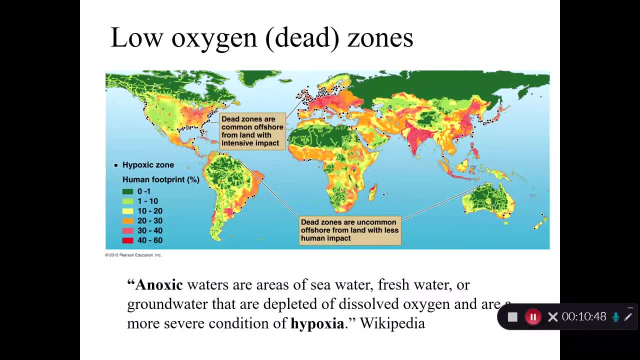 unfortunately, since all of these processes that create more reactive nitrogen are increasing in the landscape, right, we now have more and more dead zones occurring globally and associated with that, the low levels of oxygen and these die-off events, And so you can actually have affinity with a lot of seems like these are the things that the 1600s of the 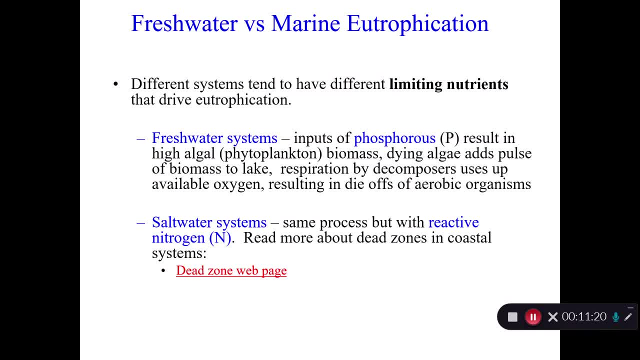 19th-century's coming up in terms of anoxic conditions, right, or even in hypoxic conditions. Now, why are these two groups? Why did we talk about both phosphorous and reactive nitrogen? It's important to think of those two as separate, even though the process of eutrophication overall 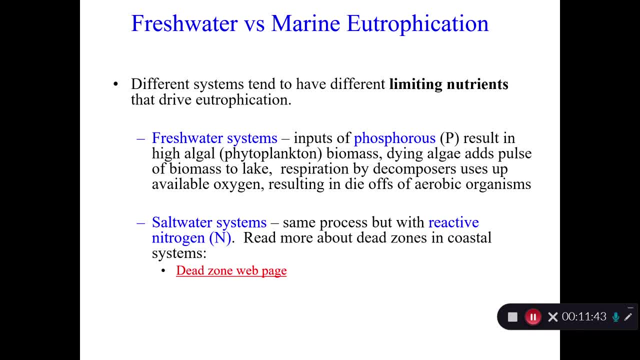 impacted. So in freshwater systems they tend to be phosphorus limited, and we'll talk a lot more about this in this class. but the main thing that it means is that, hey, if I want a lot more algae to grow in my lake, if I add phosphorus, a lot more algae will grow, So it is the nutrient that. 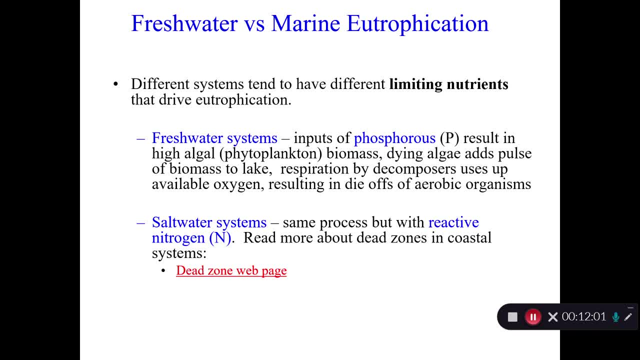 tends to limit phytoplankton growth, population growth. So phosphorus tends to be the limiting nutrient in freshwater systems as opposed to our saltwater systems. Our marine system tends to be our reactive nitrogen. That's why what we do here in Illinois right when we put nitrogen on our 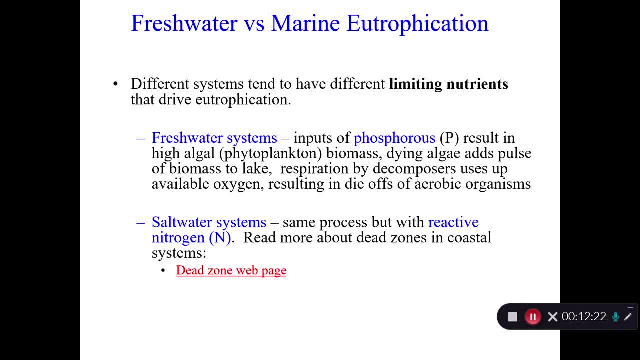 fields and then it ends up in our streams, in our lakes. eventually it gets down some of it to the Gulf of Mexico and when it hits that marine system it will cause that eutrophication event that causes the Gulf. 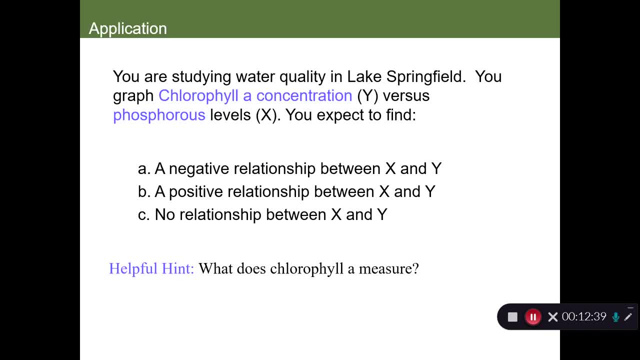 Okay. so let's take a step back and see if we can answer a question based on what we've just learned about eutrophication. So, a little bit closer to home, we want to go and study Lake Springfield because you know it's nice to be out on our boat and take a water sample. So we do that and we're. 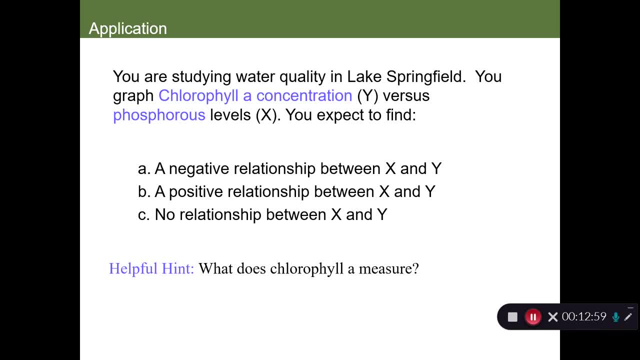 doing that over time and as we get these water samples, we measure two different things in them. One is, we're looking at um absorption for chlorophyll a, and then we're also measuring the phosphorus levels in the water. 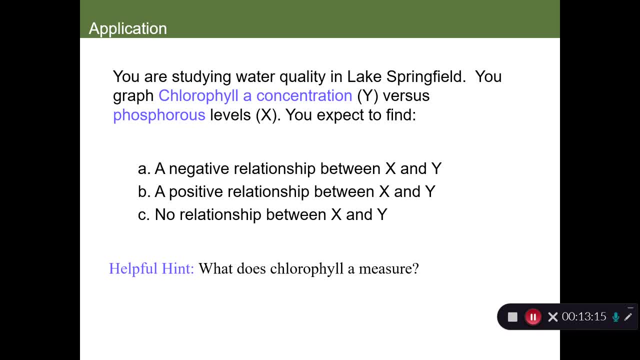 And so I have a lot of different data points. So, going in, I'm going to make a hypothesis as to what relationship I expect to see between the phosphorus level in the lake and the chlorophyll- a- excuse me- concentration. So which of these do you think is correct? Do you think you would find a negative relationship? 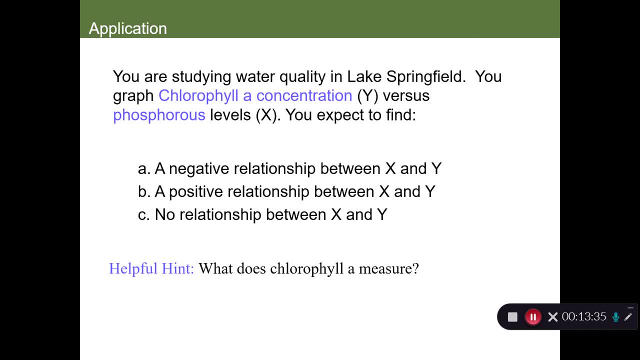 between x and y positive? Or do you think you would find a positive relationship between the phosphorus level in the lake and the chlorophyll a and the chlorophyll a in the lake? And one thing, I put it at the very beginning: what chlorophyll a measures. So, uh, think about what would have chlorophyll in the lake, right? 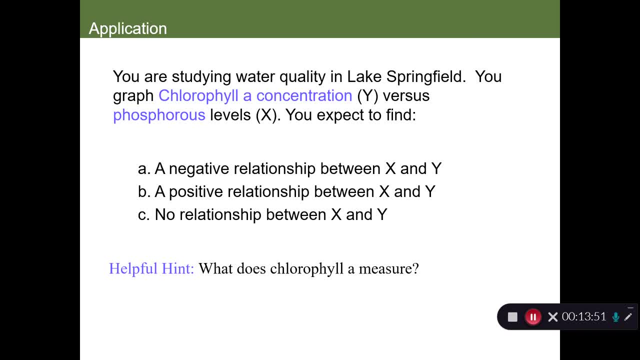 Uh, and that will help you, uh, figure that piece out. Pause it, see if you can come up with an answer, uh, and then we'll talk about it on the next slide. So hopefully you answered. oh, it's going to be a positive relationship, right? 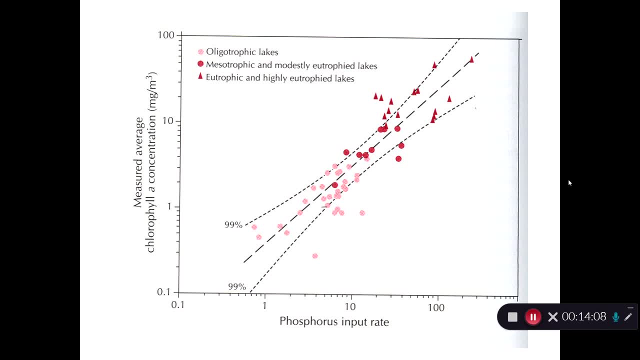 Because we're going to be talking about chlorophyll in the lake. As we have more and more phosphorus coming into this lake, you'll have more and more phytoplankton growing. I could measure my phytoplankton by seeing how much chlorophyll a is in my water. 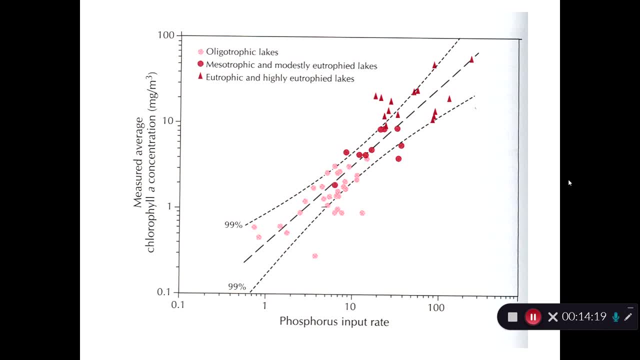 Uh, and so I should see a positive relationship. Okay, This is just showing you that, yes, we do actually see positive relationships between: on the x-axis, here, phosphorus input rate and on the y-axis, here, the average level of chlorophyll a. 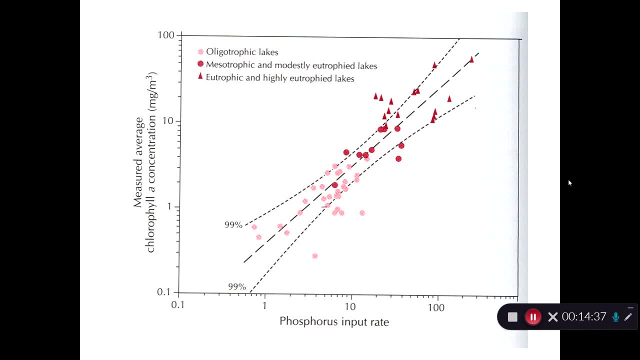 So, uh, this is just showing you that, um, that's measuring the phytoplankton levels. Now, this isn't data from Lake Springfield. What this is actually is from, uh, a cross study of a lot of different lakes. 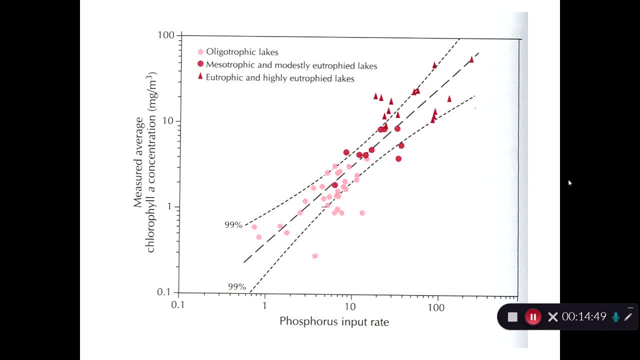 Some lakes that have much higher phosphorus inputs than other lakes, right, And so what we can see is, as you have those higher phosphorus levels in the lake, they're positively associated with higher levels of phytoplankton. Okay, That's it. Hope you understand eutrophication now.